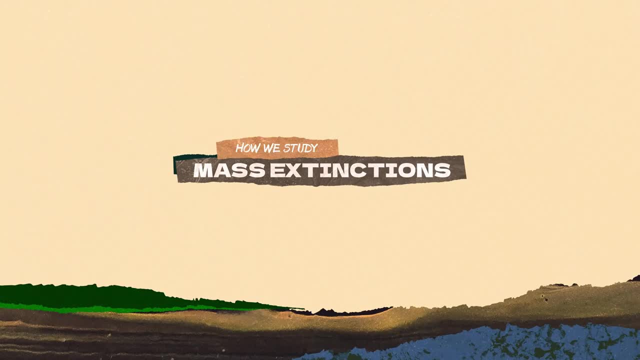 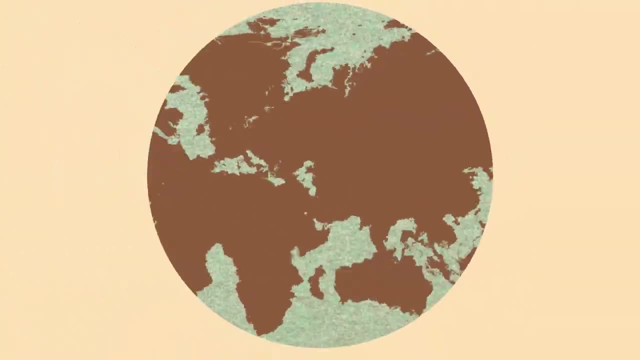 Geology is a giant puzzle. In fact, the Earth's land masses, through tectonic plate motion, have been rearranging themselves since the dawn of time. We try to put the pieces back together to understand how they were arranged all those millions of years ago. 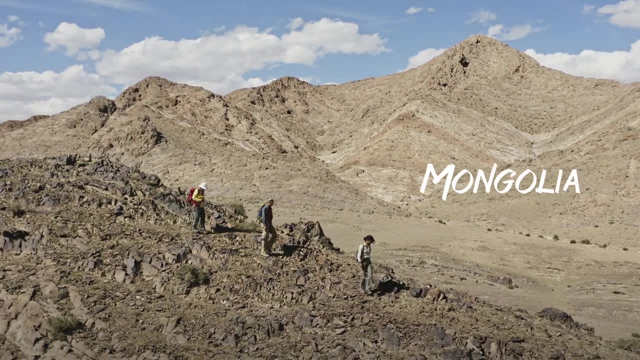 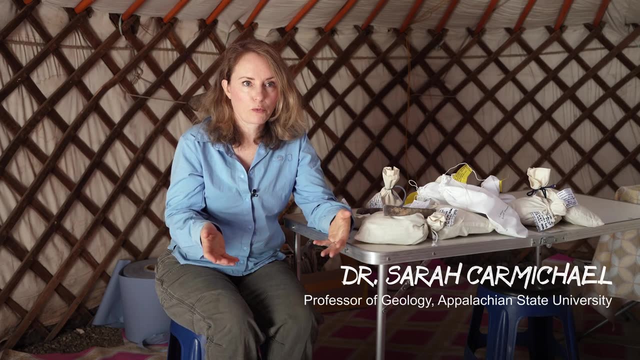 So we're in Mongolia to study this mass extinction. Mongolia is a really unusual location compared to most of the places where we've done work previously. Mongolia, even though it is one big land mass today, used to be a series of small islands. 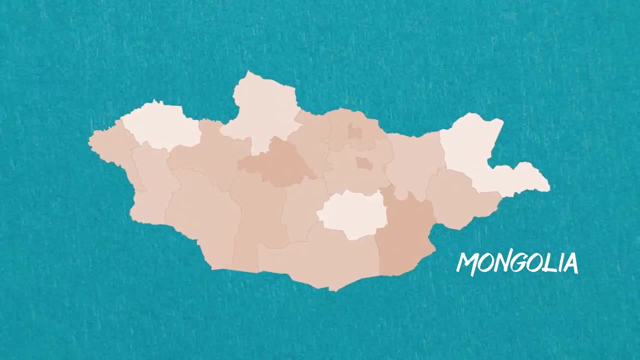 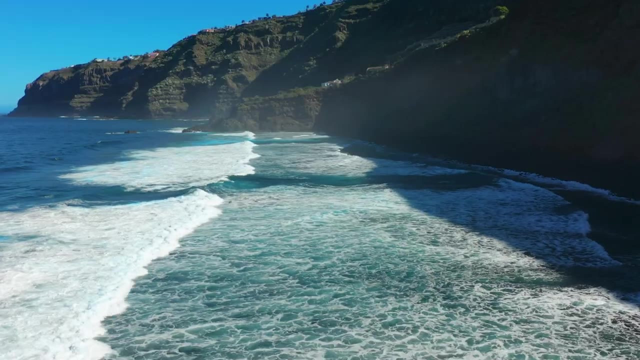 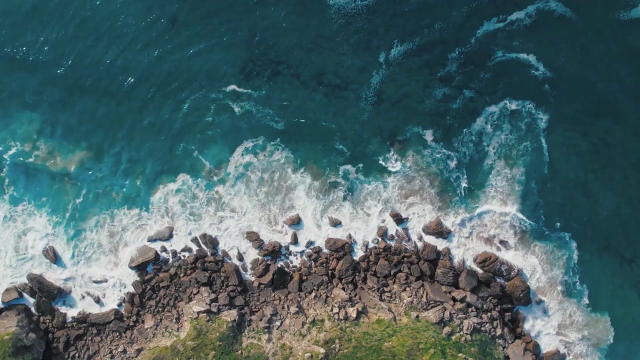 And they all got piled on top of each other into one big amalgamated unit. So if we can study this mass extinction on the coastlines of these little islands versus the coastlines of huge continents, we're going to get a better sense of what animals were living and how the extinction may have affected these animals. 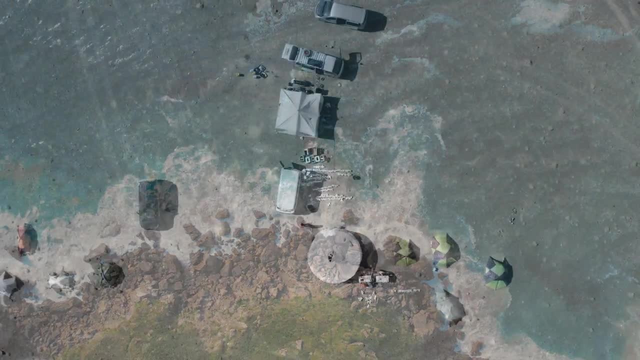 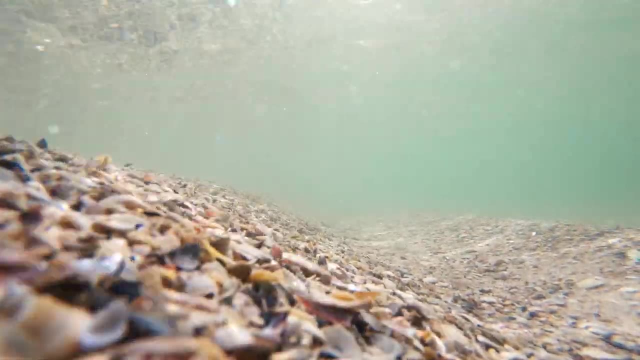 Geologists studying mass extinctions usually focus on areas that used to be under the sea. Over the years, as organisms die, volcanoes erupt and rivers wash sediment into the oceans. these slowly sink down to the ocean floor, forming deposits that we see as layers of rock or strata today. 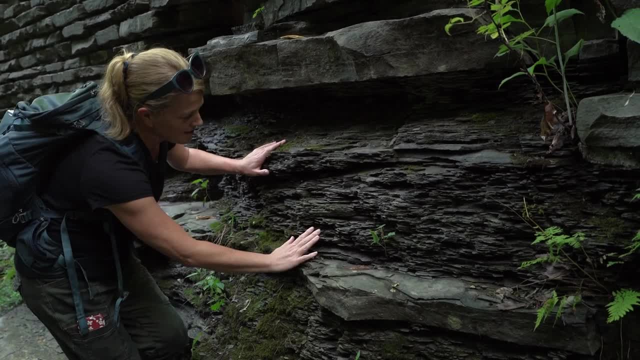 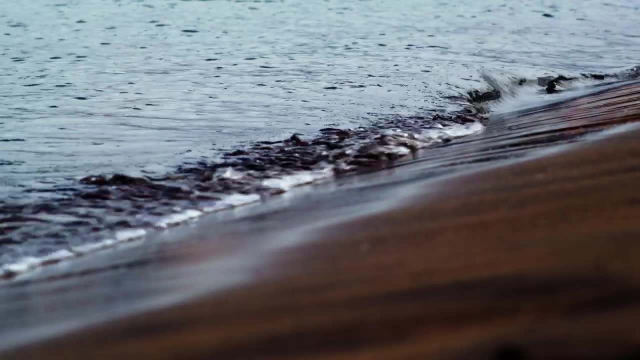 They're like pages of a book telling us what happened all those years ago, During the time period we're studying here, the late Devonian. we're looking at areas that would have been made up of shallow parts of the ocean near land, Just like today. that's where much of the marine life was from. 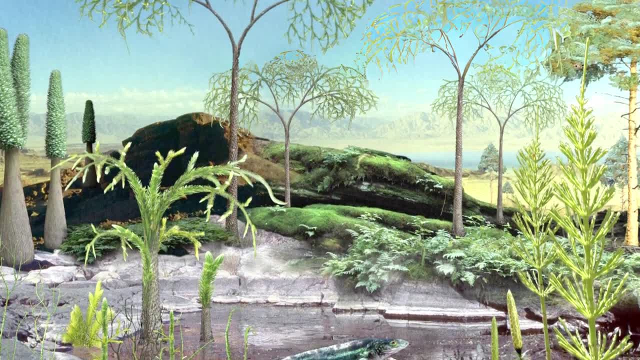 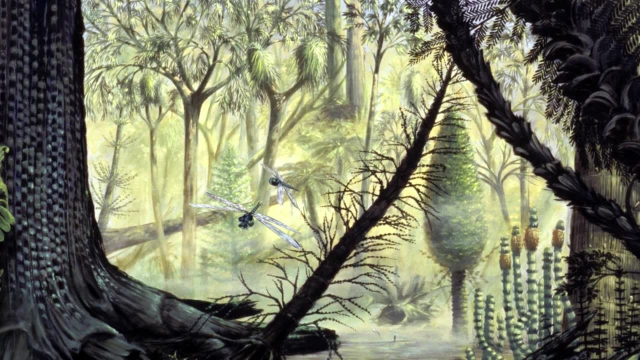 During that time, land was made up of very small parts of the ocean, Land-based life was just starting out, Organisms were just exploring terrestrial ecosystems and forests were first developed. The study of mass extinction takes place on lots of different scales. 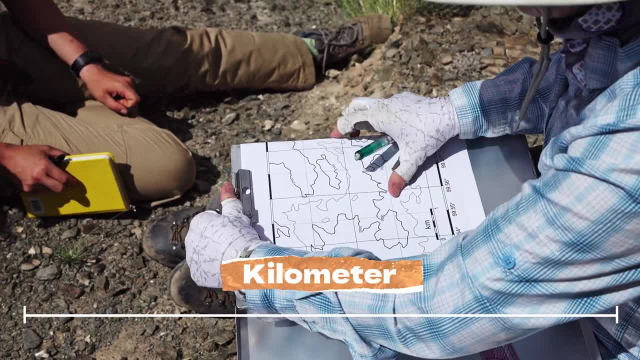 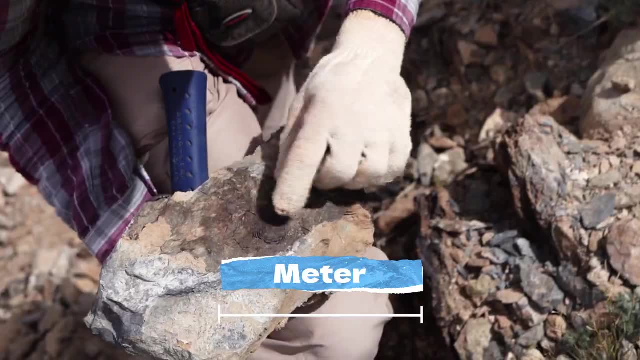 At the kilometer scale we have people doing large-scale mapping and piecing together how the land moved over time. And at the meter scale, geologists are finding out exactly how to piece together the time periods from the rocks at each location. At the centimeter scale we can look at each layer. 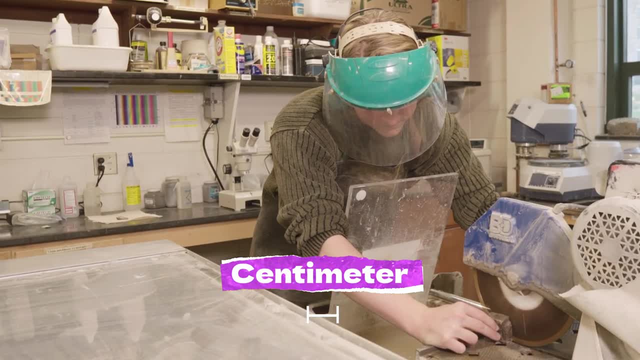 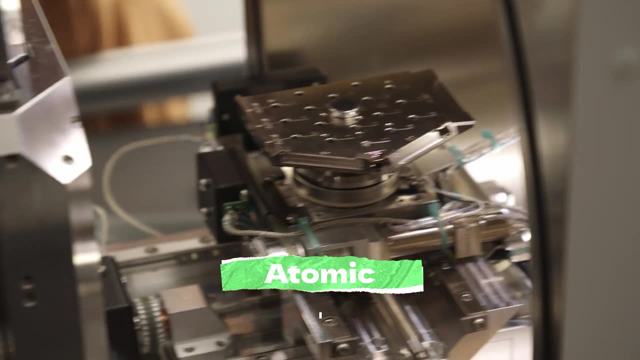 looking for changes from layer to layer over time, And sometimes there are millions of years between layers. At the atomic scale, we can see things like carbon content, carbon dioxide, cement and even the signature of what the oceans were like at that time.